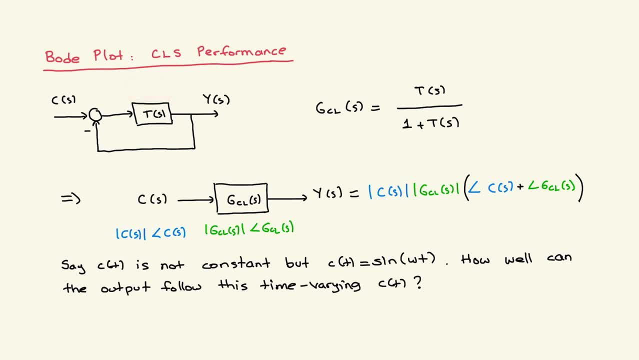 function. I am going to denote it as T. So for this un 했 feedback configuration you can write the closed-loop system like thisT divided by 1 plus T. Not that here you can have any other interesting block diagram configuration, All you need to. 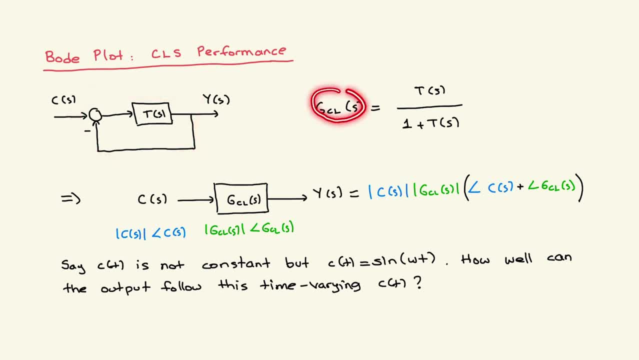 know. all you need to find is the closed-loop system transfer function. Then you can represent the field of distribution using the CM mais function. interesting block diagram configuration. all you need to know all all you need to find is the closed system transfer function, seeds ininge, so that you can represent this. 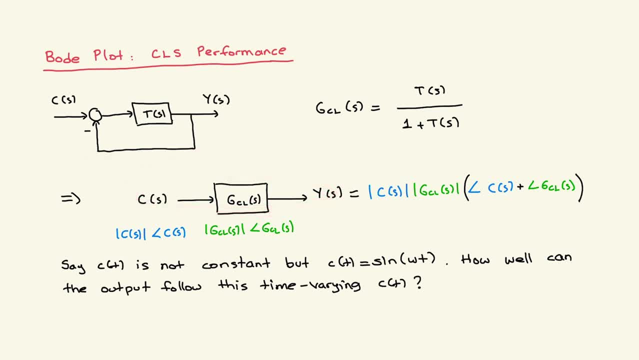 system as this basically: comment enters to your closed-loop system and your output basically goes out. now say: comment is not constant. right, we can track constant signals. either we can put a feed forward gain or a PI type compensator. but let's say we are interested to track a time varying. 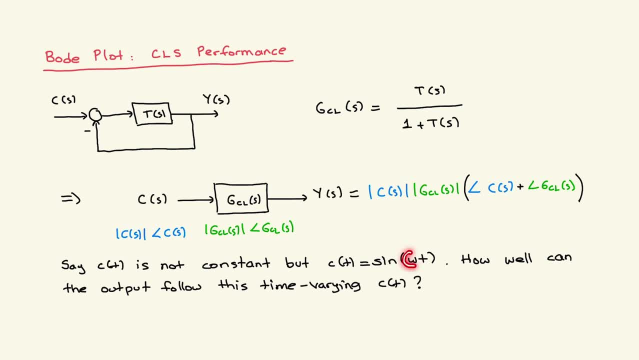 signal, and this time varying signal has a frequency: Omega radians per second. you know, basically this comment can be a combination of sine and cosines or a time varying function that can be approximated by science and cosines. all we need to know is the average or, on a ballpark, some frequency, depending on. 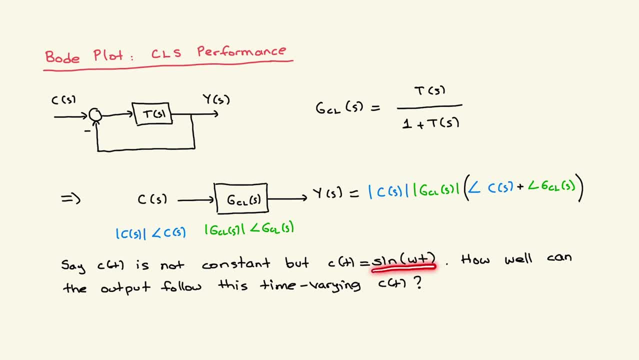 this signal. so, for the sake of the following discussion, I am going to assume sine of Omega T. so this signal has a frequency: Omega radians per second. so the question is, how well can the output follow this time? varying comment? okay, so in this case, right, this comment has some magnitude. basically, for sine, it changes between 1. 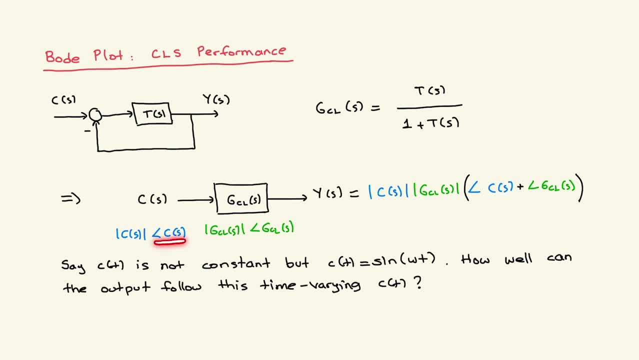 and minus 1 it is, it has some angle depending on Omega. now, likewise, this closed-loop system, transfer function, if you think, as J Omega, it depends on Omega and it also has a magnitude and the output basically of this system is the inputs magnitude multiplied by this transfer function's magnitude, plus the angle of both the input and the transfer function. now, 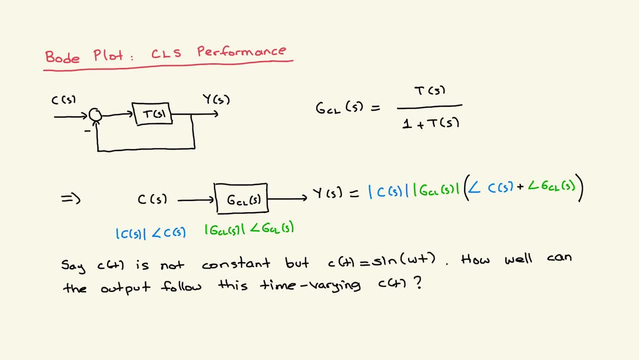 you know- I assume you know- the magnitude and the frequency of the input signal that you are applying, in this case sine Omega T. so using bode plot you can basically plot the frequency response of this transfer function and then, looking at that bode plot, you can assess whether you can track a. 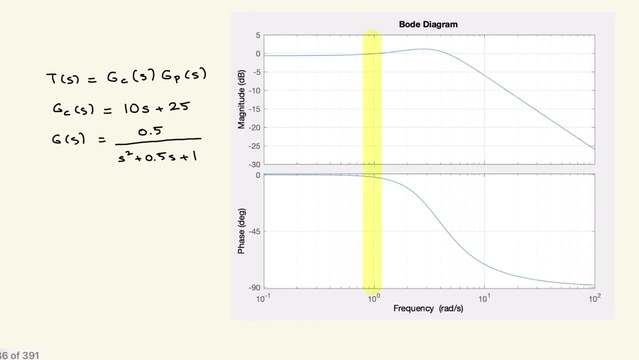 particular time, varying command or not. I will directly dive into an example. I assume you know how to sketch bode plot in MATLAB or by hand. if you want me to make a video on how to sketch bode plot, let me know. I will be happy to do so. all right, so basically, this is a in the 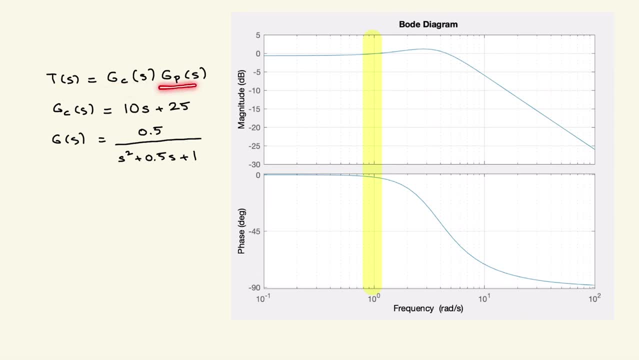 forward Loop. here is the controller transfer function multiplied by the plant transfer function. I am going to assume we have a PD type of a structure 10s plus 25 proportional derivative controller. and here is the plant. basically this controller can stabilize this system and if we look at the frequency response, 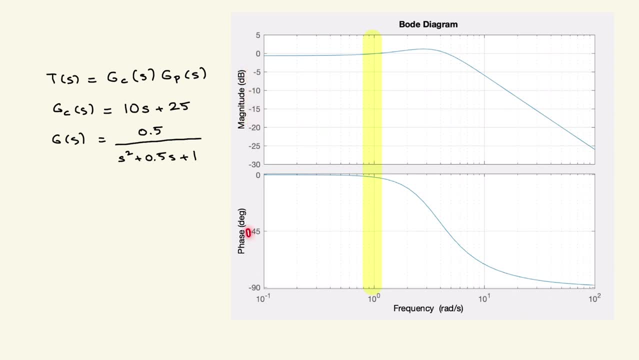 basically magnitude in decibels and phase in degrees. basically this is what we have. so this transfer functions, magnitude and phase changes as a function of frequency, for example, to perfectly track or nicely track this sine Omega T, we, when we look at here, we can see that we, we here, have zero decibels around. 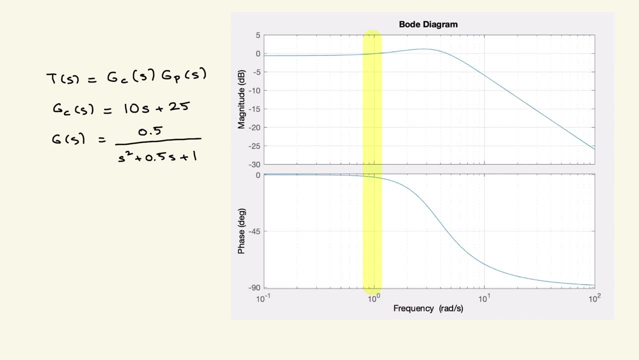 uh, one radians per second on this yellow region. meaning, and that basically the magnitude of this transfer function is one. zero decibel means one, so you can do the conversion like 20 log 10 of X is zero decibels, so here X will come out to be one. so meaning that this transfer functions magnitude at: 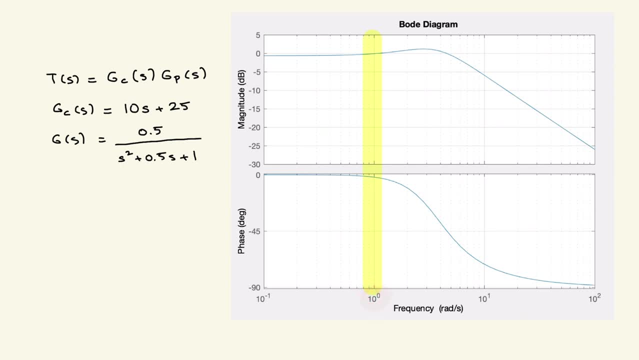 this particular one radius per second frequency is Unity, meaning that zero decibels or unity, you are not going to lose anything in magnitude at the output if you apply, on the other hand, a 0.1 radians per second, basically sine of Omega 1 T in this case. 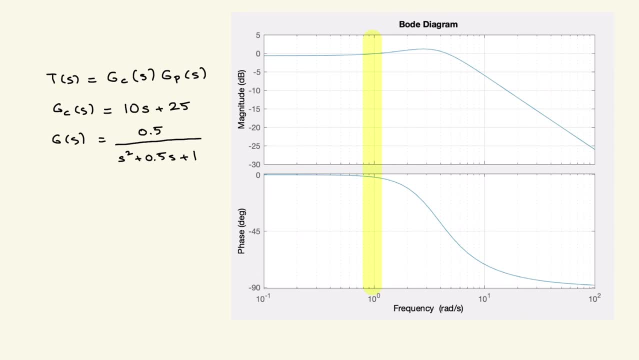 are going to lose a little bit. it is not zero decibel, you are going to lose a little bit in magnitude. now, if we look at the phase, there won't be phase shift at basically 0.1 radians per second. there will be a little bit phase shift. 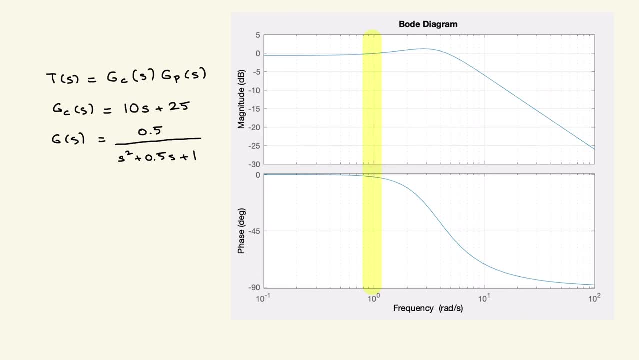 it is not notice, it won't be that much noticeable or we can ignore that. so we can assess that when we apply 0.1, we are going to lose a little bit in magnitude and we are not going to have any phase shift when we apply one radians per second sign. 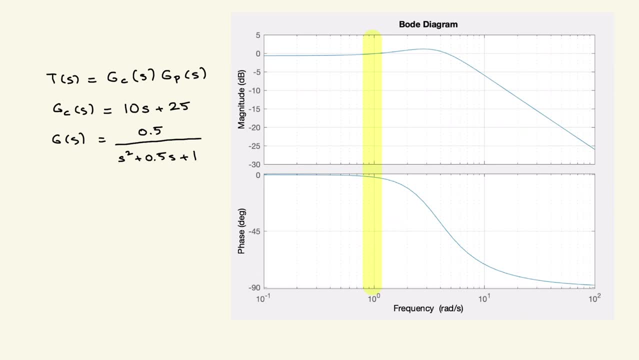 basically sine of t. we are not going to lose anything in magnitude. we are going to have a phase shift. if you apply anything more than that, for example, let's say 10 sine of 10 radians per second, we are going to lose a good amount of amplitude and we are going to going to 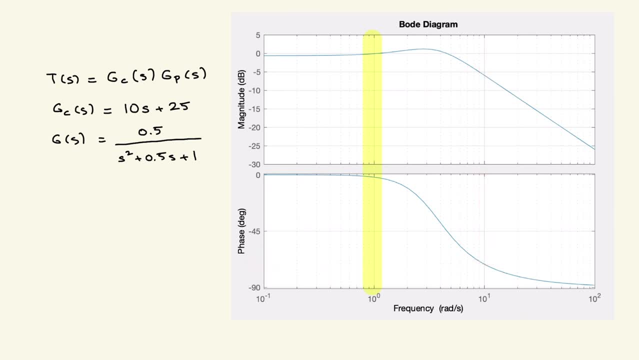 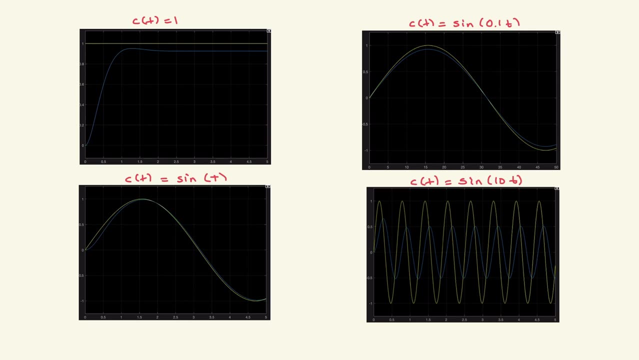 have a phase shift of close to minus 60 degrees. all right, first of all here are some plots to make our understanding better. when we apply a command of one with this controller- we could not able to track much with PD- there is some steady-state error we can directly calculate. 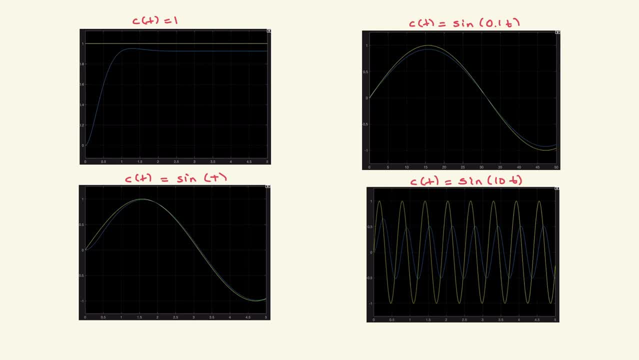 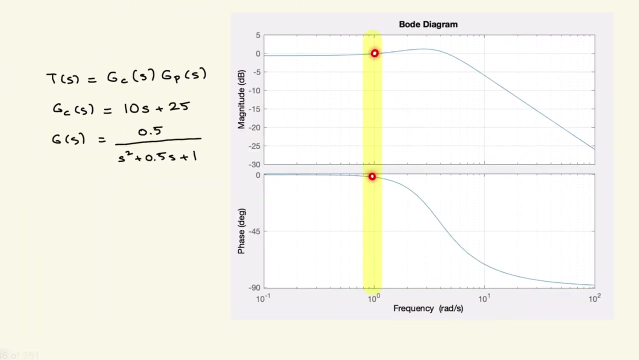 this by the steady-state error analysis. there are videos about that. there are also on my channel videos about different compensator types. you can also take a look at those like controller design or PID type of videos. now, when we apply sine of t right, we are here basically, we are not basically losing. 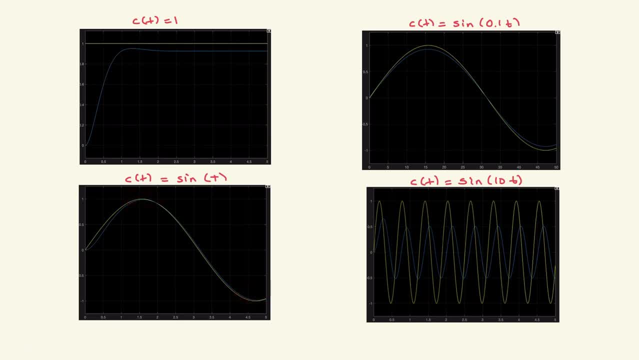 anything here. by the way, yellow is the commands that we apply this C of t and blue lines are the output responses in all figures. so this is the output. this is the C of t as expected. we can almost perfectly be nice to follow this sinusoidal signal when we apply 0.1 t. right, I mentioned we 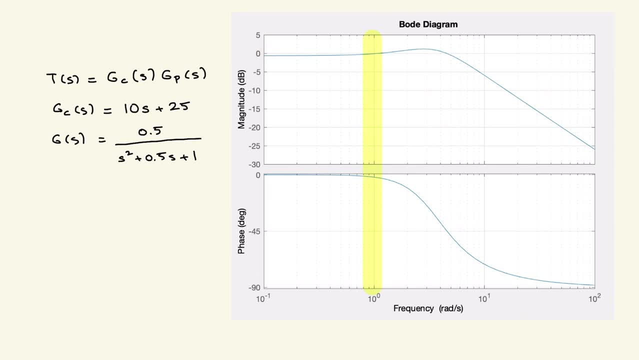 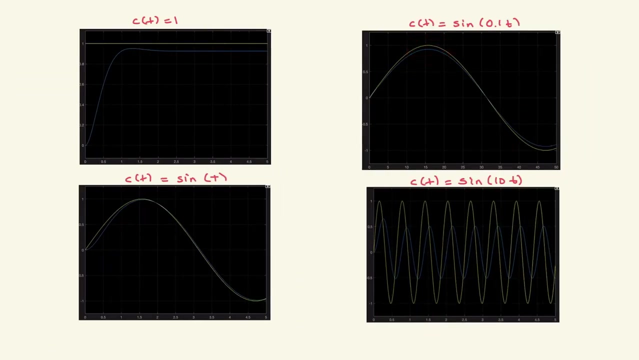 are going to lose a little bit. we are looking for zero decibels to perfectly track in magnitude and we are looking for no phase shift. and when we are applying a sine 0.1 t, we are losing a little bit in magnitude, as expected from from the body magnitude plot. there is no phase shift. now, when we 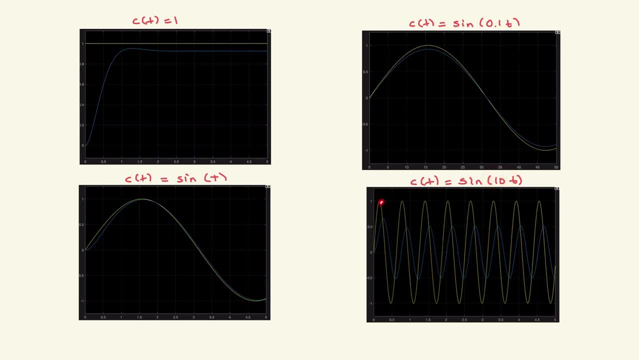 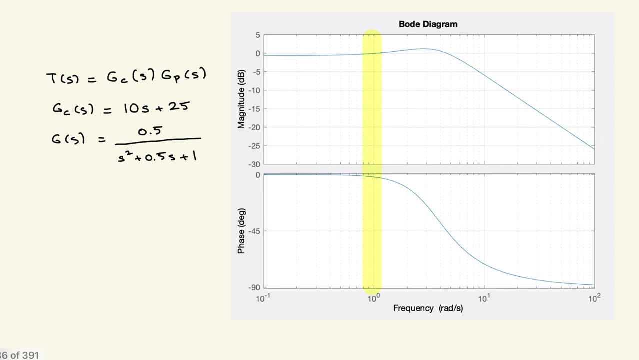 apply sine of 10. right, this is C of t. again, this is the blue is the Y of t. we are losing L, pretty much or close to half of the signal which is also expected from this bodyplot. if you look at here, basically, here we are looking at minus 6 decibels, so minus 6 decibels if you convert to. 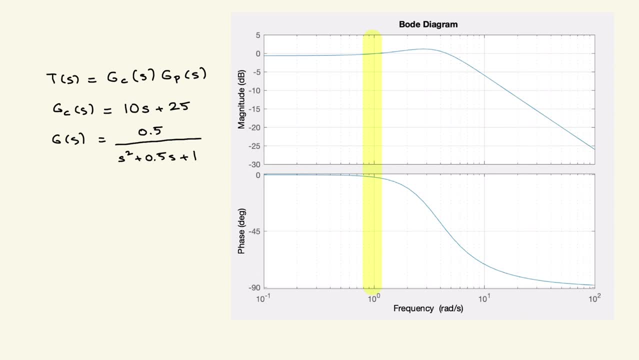 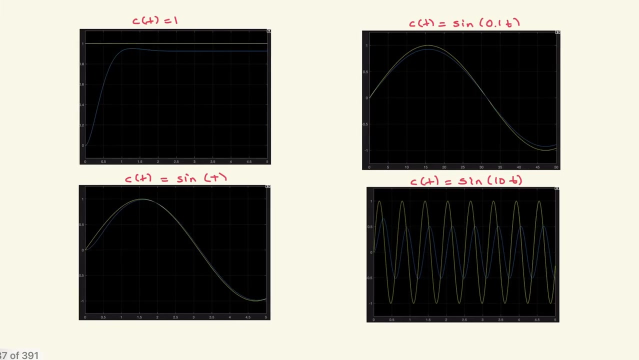 basically, if you convert our regular language log, 10 of X minus 6, if you find X, you are going to lose. it will be 1 over 1 over 2, so you are going to lose half of the signal and uh, And you can directly see phase shift, expected phase shift. 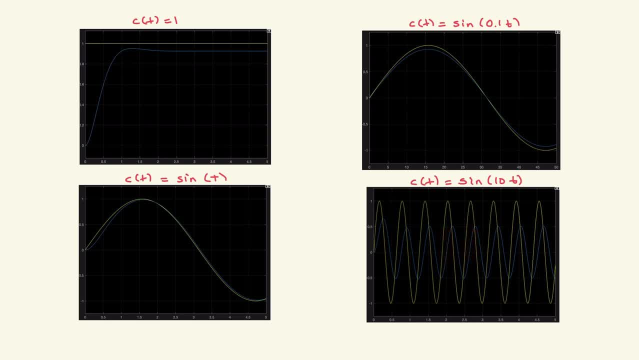 So for this example, first example- we can say that we can perfectly track sine of t which is expected from the body. plot Now in the following examples- I am not going to plot system or closed loop system responses as a function of time, because I hope this example tells you. you know once you look. 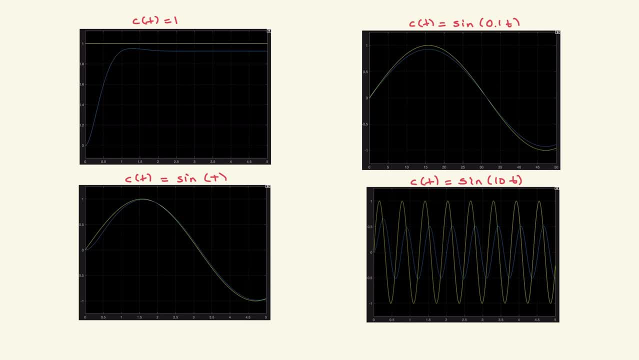 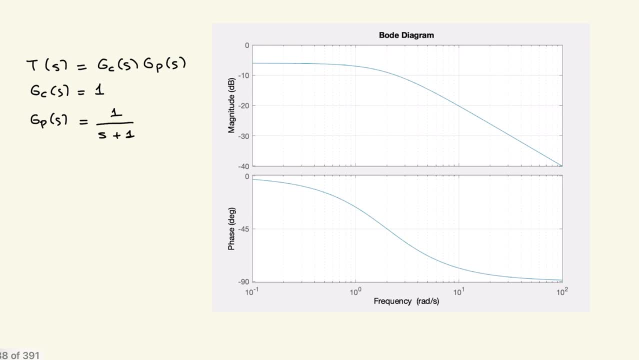 for the region on the body plot that has zero decibels and no phase shift. you can perfectly track sinusoidal signals. All right, so let's look at this example now. g of s is one, gp of s plant is one divided. 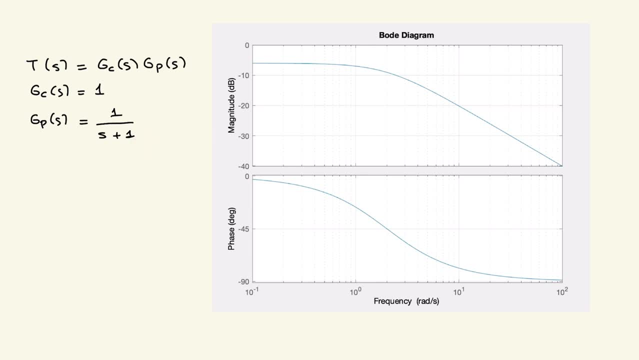 by s plus one. If you look at the body magnitude plot, We never hit zero decibels, So this is around minus six. So if you basically apply a sine of t, sine of omega, t with omega belonging to somewhere, this region between 0.1 to one, you are going to lose half of the signal. 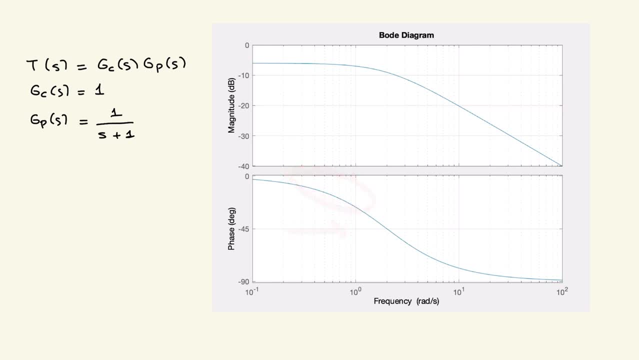 And as you approach the here, you are going to have more and more phase shift. So So it is useful, right? I mean it is useful to plot the closed loop systems, transfer functions, body plot to assess you know how well you can track time varying commands. 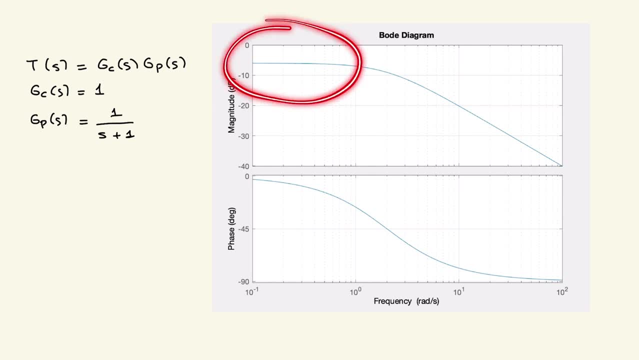 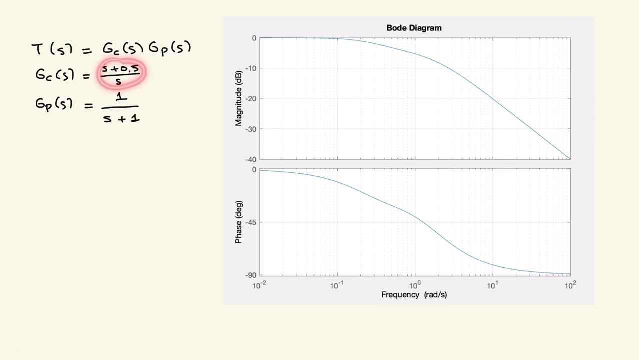 Now, in this case, you cannot. we have a huge loss here. we don't have zero decibels. Now let's change this controller to a PI type of a controller. With this PI controller, you know, we could be able to track constant commands. 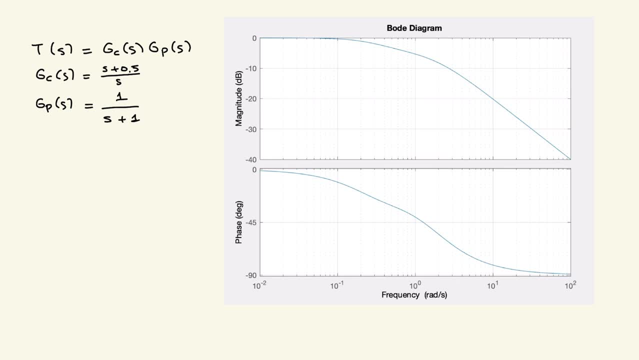 And you can see here we have zero decibels And we can also track a set of time varying commands. right, Let's write: C of t equals to sine of omega t. So let's look at the magnitude plot Up to here, basically- I can go a little bit further up to here- basically for omegas belonging: 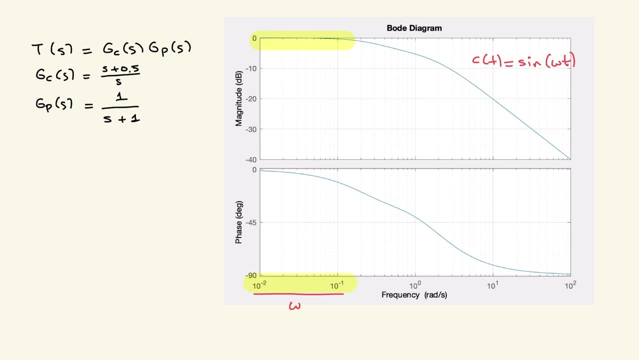 to this range. I am not going to do that. I am not going to lose much in the body plots, you know, like transfer functions, magnitude, so that since this magnitude will be multiplied by inputs magnitude at the output, I am not going to lose anything. we can basically output magnitude wise. we can have a good match with. 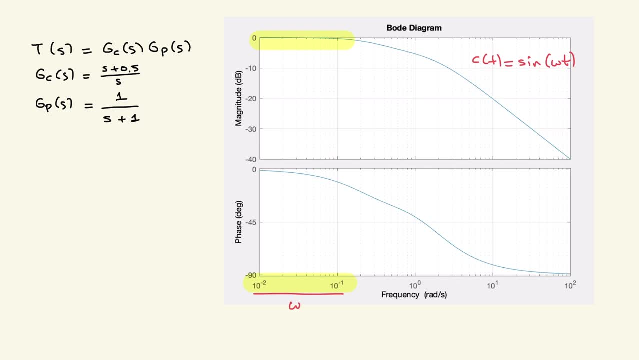 the input. Now, if we look at the phase, well, I am going to have, I am going we are going to have kind of a noticeable phase shift after maybe 0.08. this point, if it is fine, you know, you can go up to. 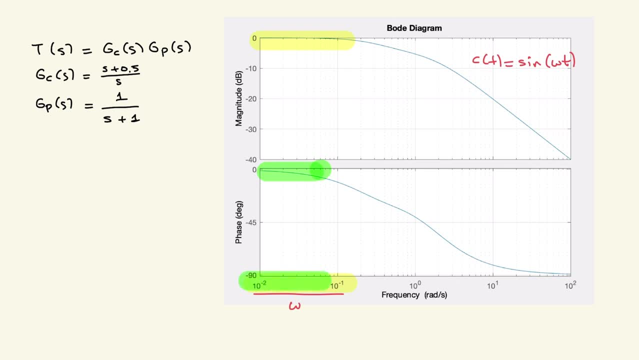 here. basically look, taking the intersection between these two regions, we can say that if omega of the input belongs to this, I can say 0.01 to 0.08 radians per second. I could be able to track sinusoidal signals well. 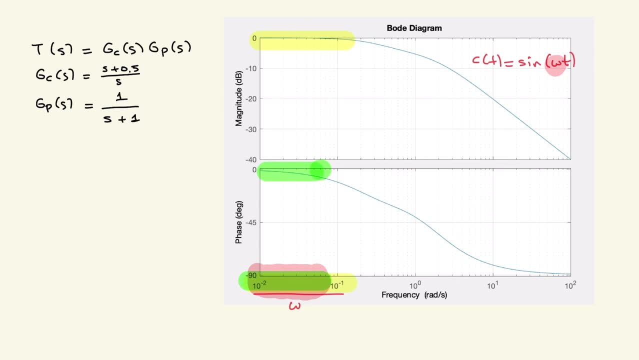 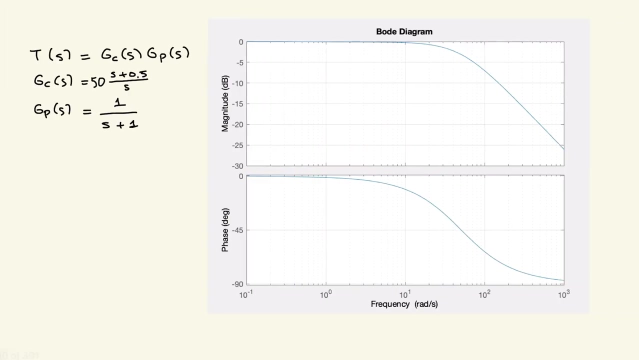 Okay, And this is you know, we know, PI compensator allows us, if it allows basically comment following performance of constant comments and it also allows tracking of time varying comments up to a point Now. next, basically I am adding again 50, basically I am trying to increase so called.